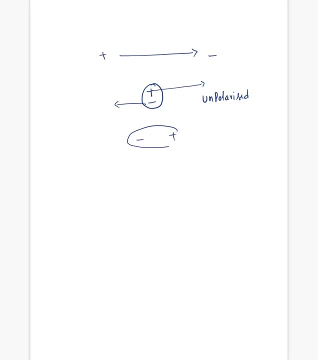 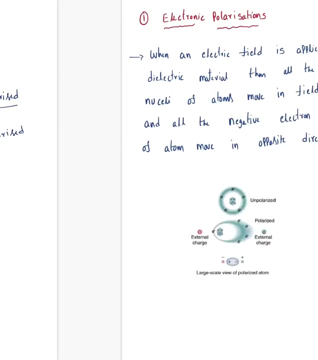 become a polarized molecule. So the process of producing dipole moment, or the process of producing a dipole, or the process of converting unpolarized molecule into polarized molecule is called polarization. So now, here we are going to discuss about. 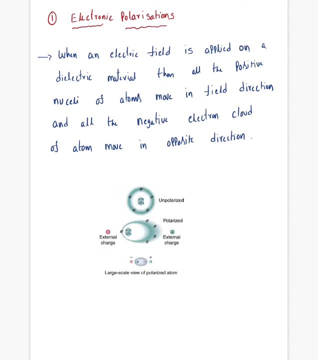 three different types of polarizations Now. the first one is an electronic polarization. So what is meant by an electronic polarization? When an electric field is applied on a dielectric material, then all the positive ions, positive nuclei of atoms, move in the field direction. 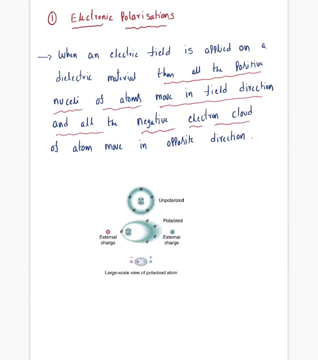 and all the negative electron cloud of the atom move in the opposite direction of the field. So this is, if you take this, this in this diagram, if you take this, the first one is unpolarized atom. means the, The nucleus is at the center and this nucleus is surrounded by electron cloud means both: 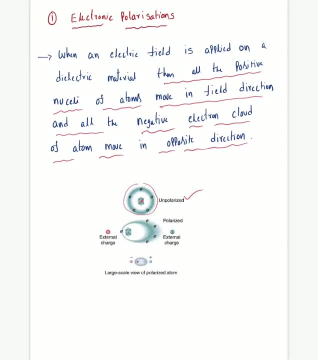 positive charge center and negative charge center. both are at the same point. So this is unpolarized atom. Now, by applying electric field, they applied electric field like this: By applying electric field, the positive nuclei of atom is moving in the field direction, like 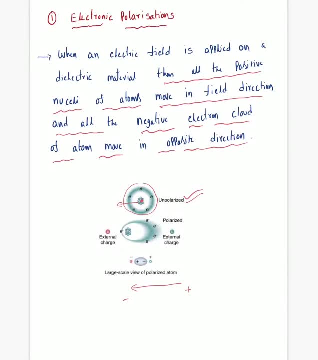 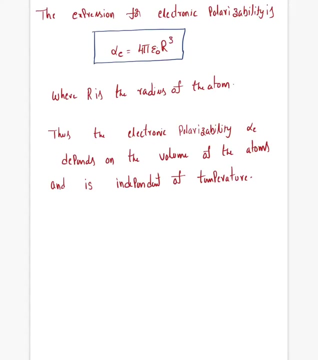 this and electron cloud. all the negative charged electron cloud is moving opposite to the field direction. So this type of polarization is called electronic polarization. Now the expression for the electronic polarization is mentioned here like this: alpha e is equal to 4 pi epsilon. 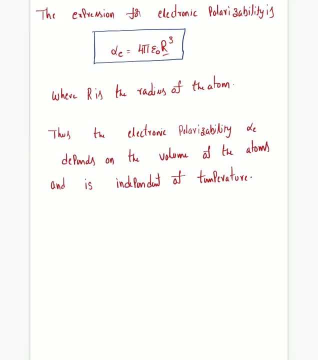 naught r cube. Now here this r is called the radius of the atom. So the electronic polarizability alpha e depends upon the volume of the atom. it depends upon the volume because 4, pi epsilon naught r cube, r cube represents the, here the volume of the atom. 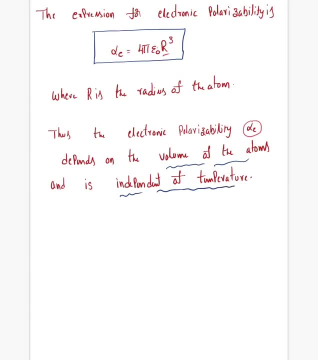 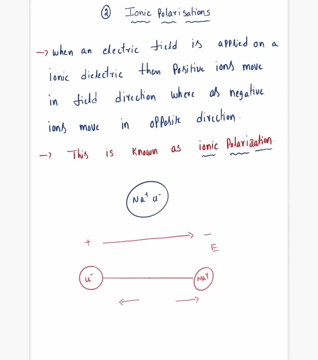 And it is independent of the temperature. So electronic polarization does not, does not depends upon the temperature of the material, A temperature, what we are applying, the dialectic material. So this is about electronic polarization. now the second one is ionic polarization. in this, when electric field is applied on 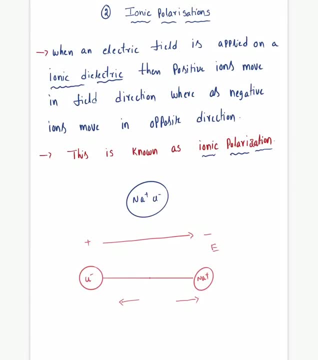 a ionic dielectric material is applied on a ionic dielectric material, then positive ions move in the field direction And whereas the negative ions moving the opposite to the field direction. So this is known as ionic polarization. So generally we will take one example, that is NaCl molecule. 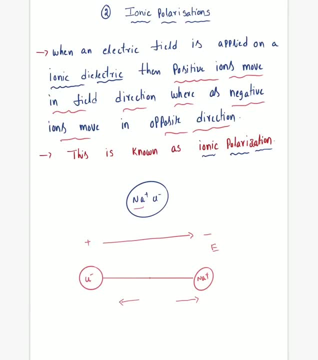 NaCl molecule is made up of Na plus ions and Cl minus ions. So in unpolarized ionic molecule both positive charge center and negative charge center, both are at the same point. So by applying electric field the Na plus ion will move. 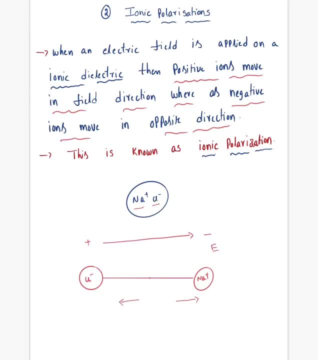 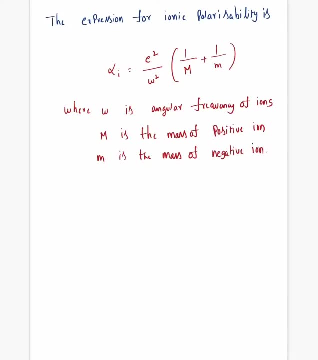 in the field direction and Cl minus ion will move opposite to the field direction. So this type of polarization is called ionic polarization. Now, the expression for the ionic polarizability is expressed like this, or mentioned like this: Alpha i is equal to e square by omega, square into 1 by M. 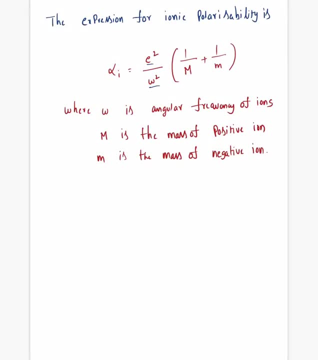 capital M plus 1 by small m, where omega is the angular frequency of the ion and capital M is the mass of the positive ion. Here we make an expression like Na plus and small m is the mass of the negative ion. nothing but like, example, Cl minus ion. So this is about the ionic polarization and the 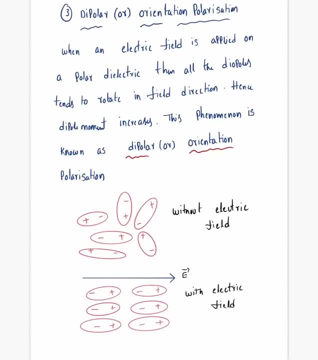 third one is the dipolar, or orientation polarization. So in this when an electric field is applied on a polar dielectric material. In previous case we applied electric field on ionic dielectric material. Here we are applying electric field is on polar dielectric material. Then all the dipoles, because 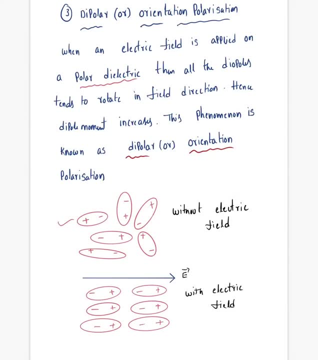 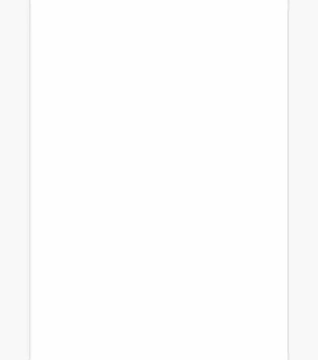 already. already, they are all polarized here. we can see here: all the dipoles, all the all the molecules are polarized here. Then all the dipoles are tend to rotate towards the field direction. hence the dipole moment increases because already polarization is there. So then, what happened now? but they are oriented in. 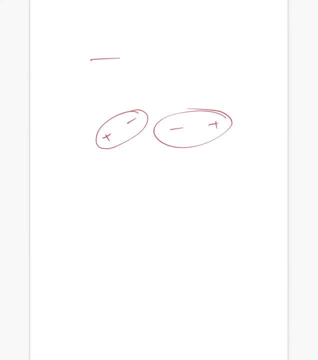 different direction. like this, they are oriented in different direction. So when you apply electric field from positive to the negative, the negative charge will attract towards the positive side and positive charge will attract towards the towards the negative side. So in this way, the dipole will be oriented like this: